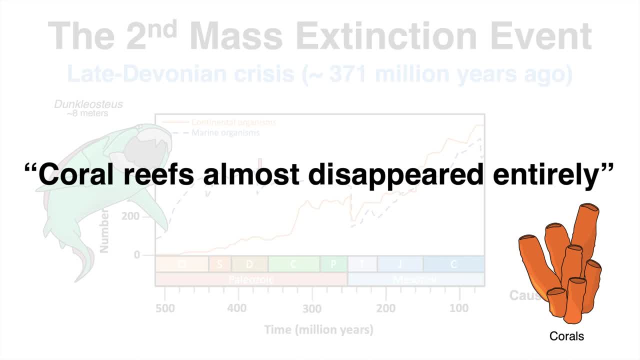 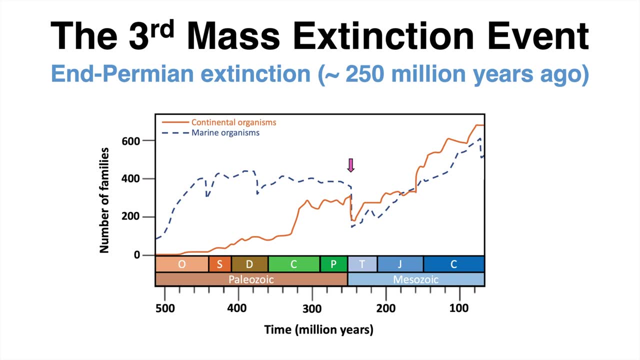 were hit especially hard, which led to a significant dying of coral reefs in the ocean. The third mass extinction event was the most severe of all five. The end Permian extinction occurred around 250 million years ago. An estimated 90% of all marine species went extinct during it. 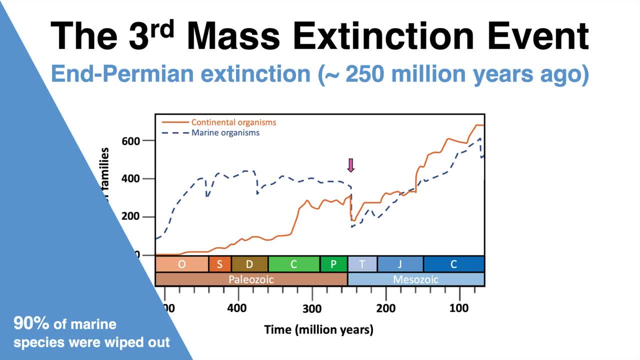 And for the first time, also terrestrial families were severely affected. Therefore, the third mass extinction event in the end, Permian, is widely known as the Great Dying. What caused this gigantic loss of organisms is still debated. It may have been meteorites or methane, but one of the most accepted theories is that the 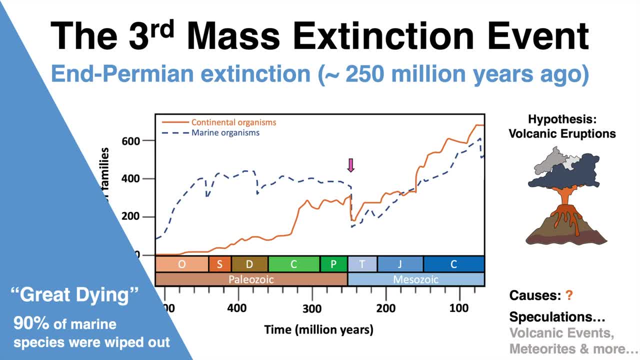 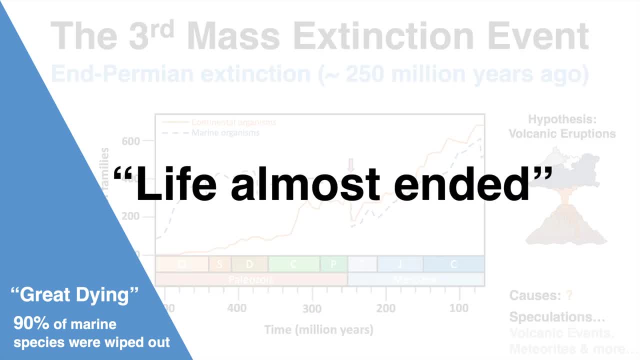 Great Dying could have been initiated by volcanic eruptions. This could have been caused by volcanic eruptions. Even though this puzzle is not entirely solved yet, we know that the era of a multitude of marine organisms ended here. Trilobites went extinct, The remarkable sea scorpions were eradicated, but terrestrial 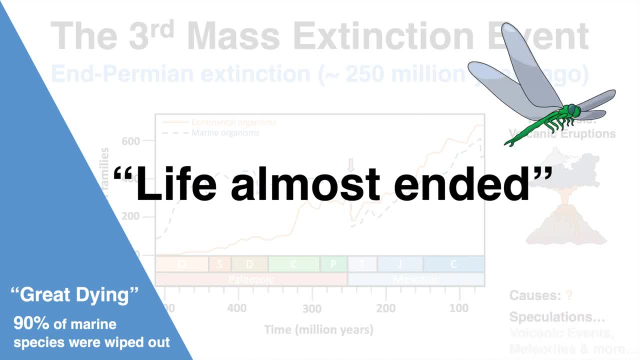 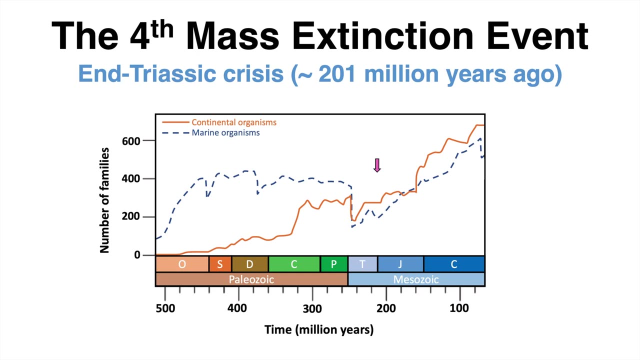 organisms were also massively affected, Even insects. It has been suggested that around 70% of all terrestrial species disappeared. Life was literally on the edge. The fourth great extinction event occurred in the era of dinosaurs and defined the so-called Triassic-Jurassic boundary. 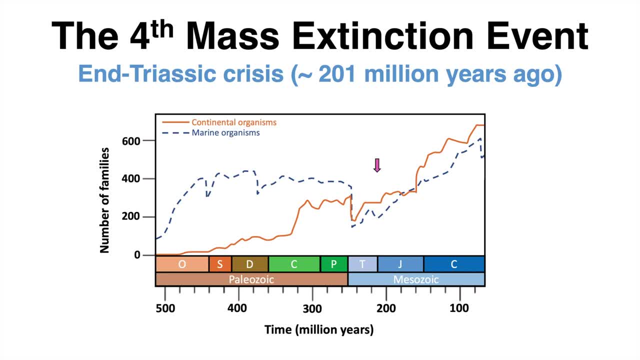 In the middle Triassic, the coral reefs had finally recovered. During that time, the marine environments were dominated by ichthyosaurs, an ensign group of large marine reptiles. 201 million years ago, the fourth great mass extinction event led to the disappearance of 75% of the species at that time. 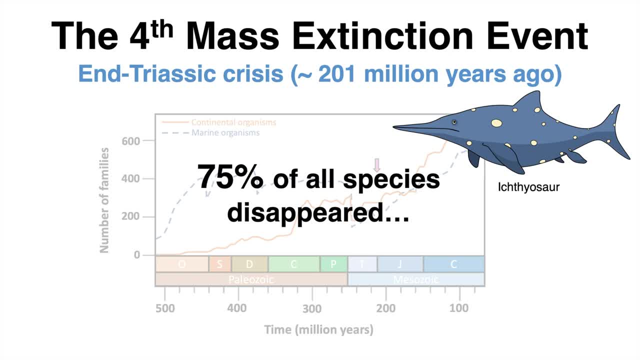 There is much evidence that the incident was caused by massive volcanic eruptions. once again, The consequence must have been a global warming period and quadrupled carbon dioxide levels that led to ocean acidification. Therefore, oceanic life was hit particularly hard. The last big mass extinction event is infamous as the end of the era of dinosaurs. 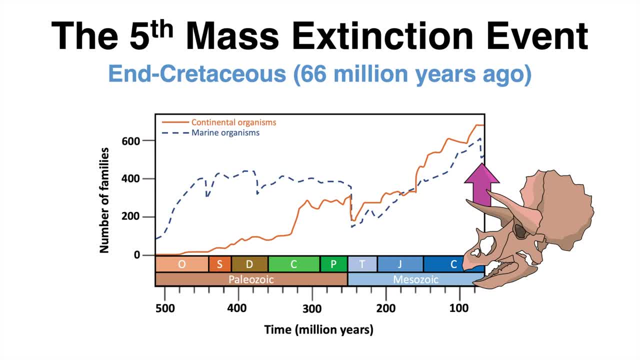 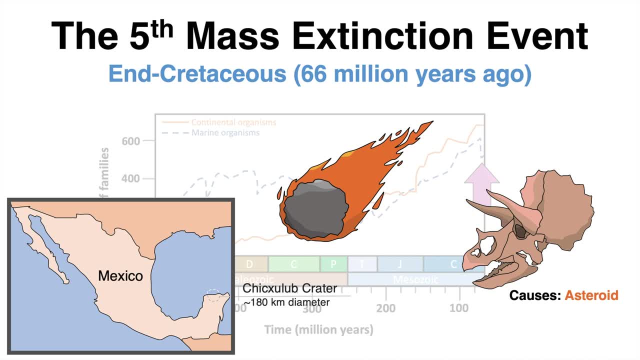 66 million years ago, At the end of the Cretaceous, a massive asteroid with a diameter of around 10-12 kilometers hit Earth. A crater almost 200 kilometers wide located in today's northern Mexico is proof of the impact. Even though the asteroid impact is the favored and well-accepted